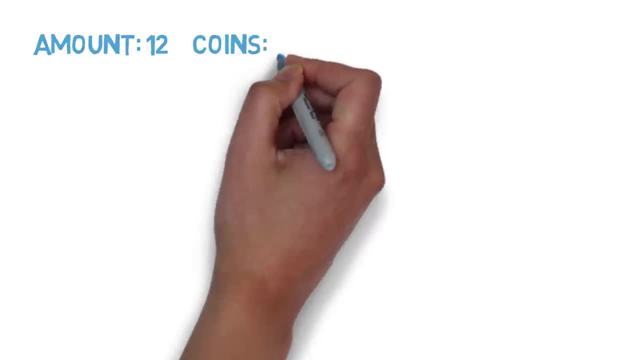 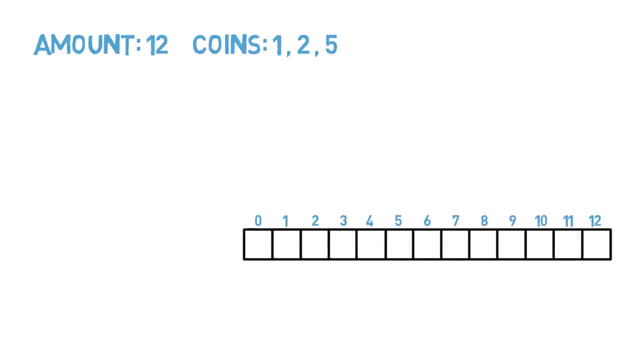 So let's look at this example. You were given the amount twelve and again the coins one, two and five. The first thing we're going to do Is create a one dimensional array: the size of amount plus one. We call this array combinations. 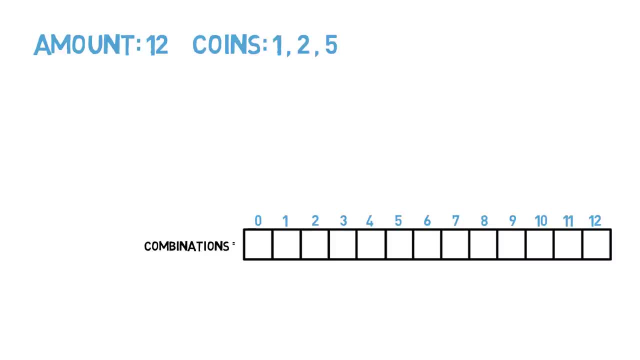 We can do this because the value stored in the array will be the total count of combinations for the different amounts. Each location in the array will correlate to an amount of money. So the location six in the array will correlate to the money amount of six. 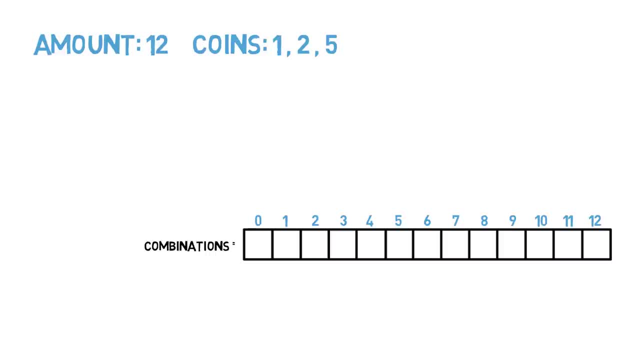 We're going to iterate through this entire array for each coin given as a parameter. The logic we use to fill this array during each iteration goes as follows: If the amount is greater than or equal to the coin value, Then the amount location in the combinations array will result in its current value plus the value in the location, amount minus coin. 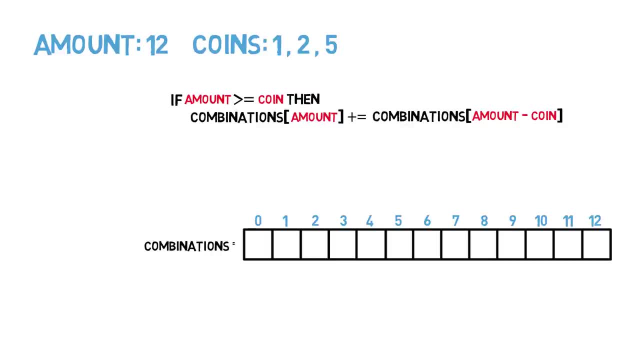 This may sound tricky, but it's really quite simple. Let's go through this example to help you better understand the logic. We begin by iterating through the entire array with coin one. The first thing we need to do is set up amount zero with the value one. 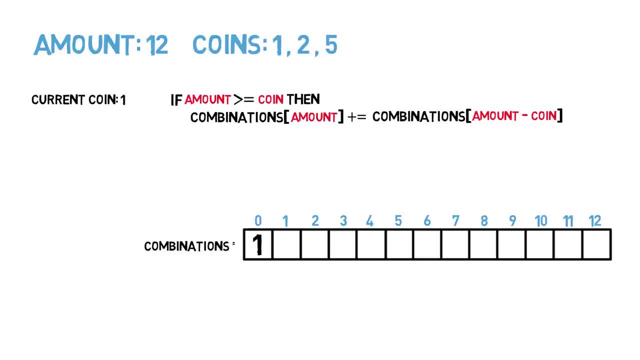 This will never change, because a coin can never go into zero. I'll explain in a second why we give it that value. Now we can look at amount one and go through the logic. One is equal to coin one, So we go through, which means there must be a combination. 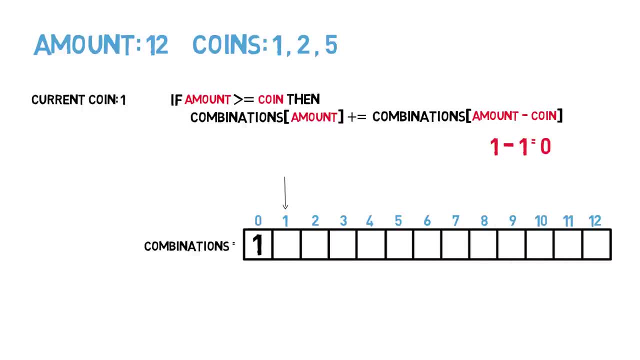 We do amount one minus coin one, which leaves us with zero. We look at amount zero to find the value one inside. This confirms a combination And this is why we created amount zero with the value one. We can now give amount one the value one, signifying a single combination. 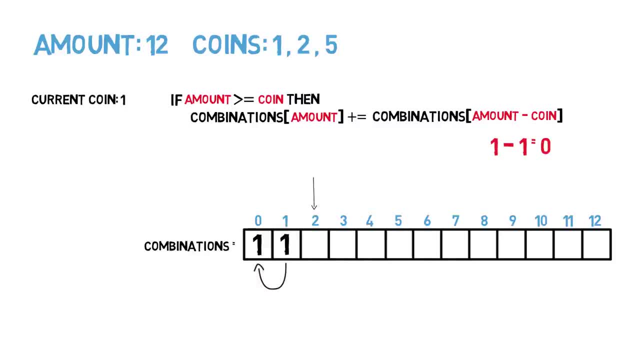 So let's move on to amount two. Two is greater than one, so we move on. The amount two minus coin one gives us one. We look in the combinations array for amount one and add it to amount two's current value, which is zero. 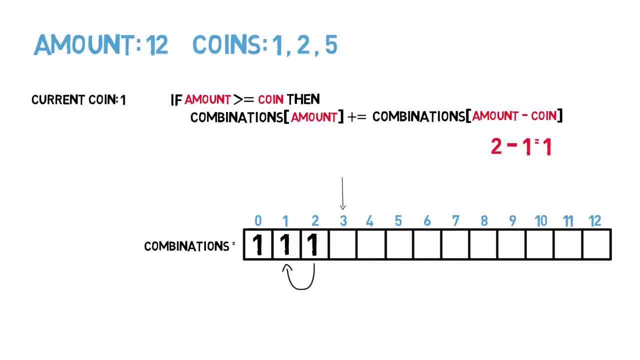 Now amount. two has one combination. Same thing happens with three. Three is greater than one, and three minus one equals two. We take the value in two and add it to three, which is currently zero. Now three has one combination. We can do this for the rest of the array and we get one combination in each. 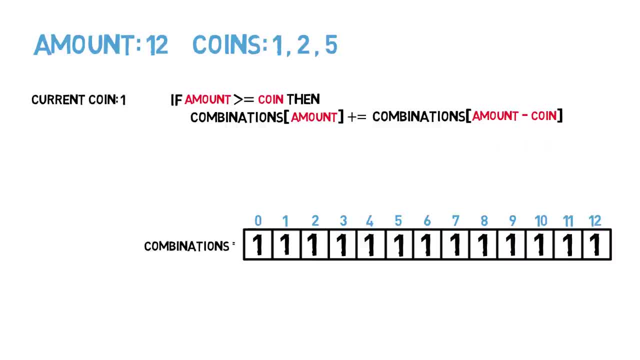 This makes sense because one goes into every amount. Since we are done with coin one, we can now move on to coin two. So now we start back at amount one. Is amount one greater than or equal to two? No, it isn't. So we skip amount one and move on to amount two. 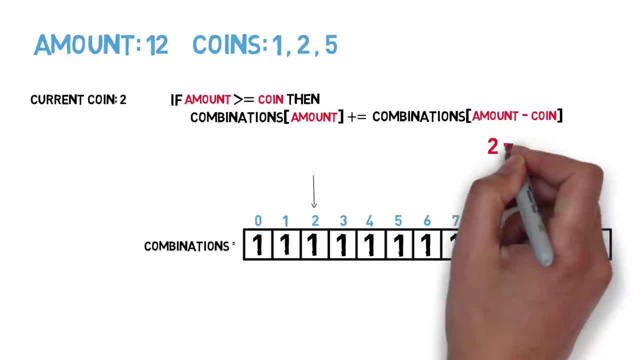 Two is equal to coin two. So we do the same thing we have been doing. Two minus two gives us zero. We look at amount zero and add its value one to the current value one. This will give amount two, two combinations. Let's look at three. 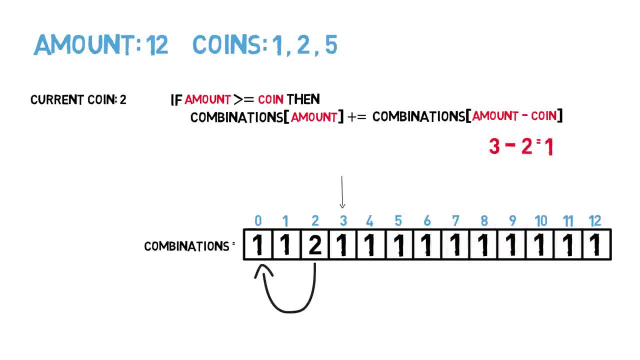 Three is greater than two, so we do three minus two, which equals one. We take the value from one and add it to amount three. This gives us two combinations. Now let's do four. Four is greater than two, so four minus two equals two. 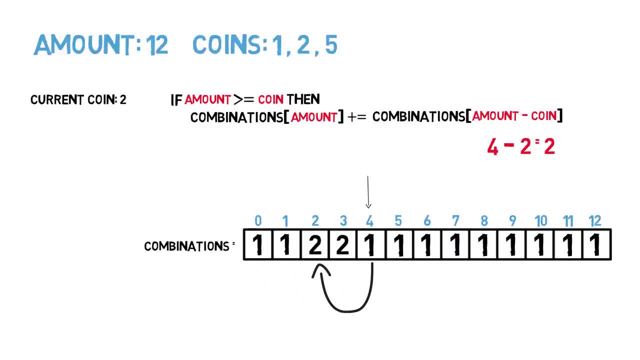 We check amount two and we add its two combinations to the value of amount four. This gives us three total combinations. If this is confusing for you, think of it like this: There are two ways to create amount two that we have already found. We are just adding another coin two to both those combinations to create four. 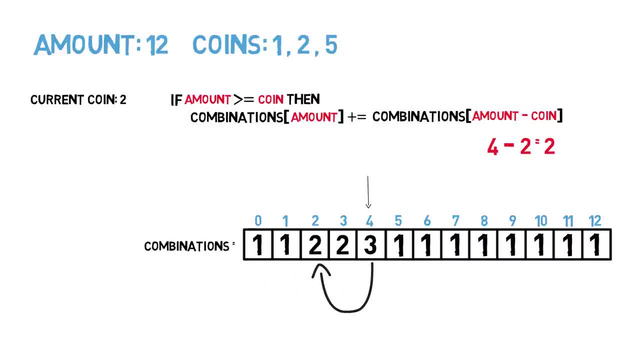 Then we have the one plus one plus one plus one And the first coin iteration, giving us three total. Now we can do this for the rest of the array And at the end of two full iterations there are seven total combinations for amount twelve. 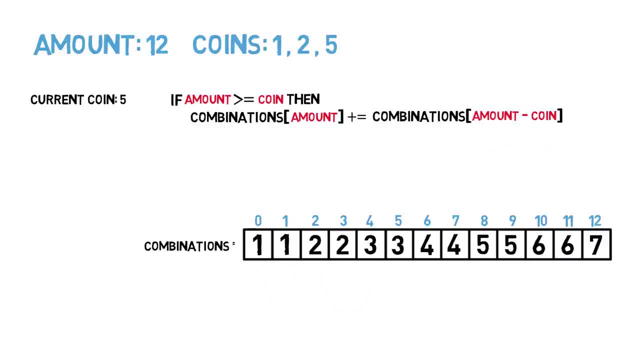 So let's finally look at our last coin five and iterate it through the array. Since coin five is greater than the amounts one, two, three and four, we can skip them. Let's look at amount five. Five is equal to five, so we do five minus five, which equals zero. 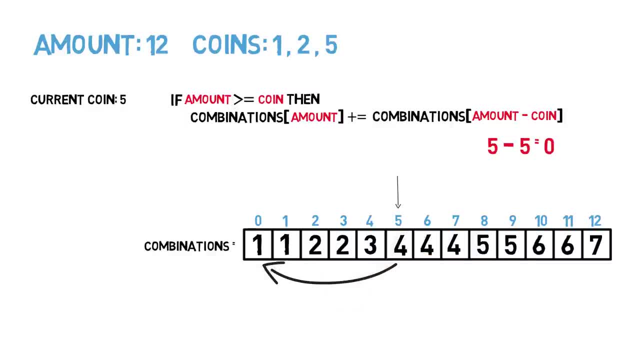 We take the value at amount five and add one to it. This will give four total combinations. We do the same thing with amount six. Six minus five equals one. We take the value in amount six and add one to it. This gives us a total of five combinations. 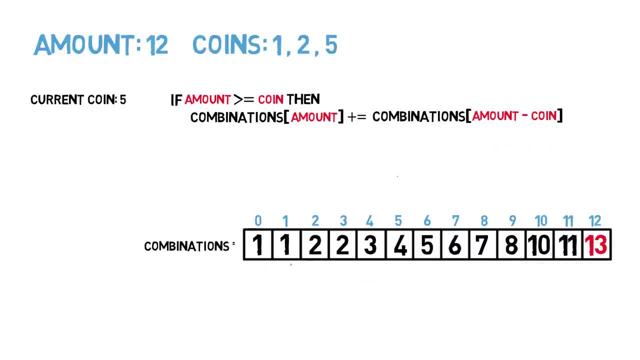 So hopefully by now you get this process. We can do this for the rest of the array to get our final results. You can see that there is a total of thirteen combinations for amount twelve And we can give this as our final output. If you were also asked to find the total combinations of any number in the array. 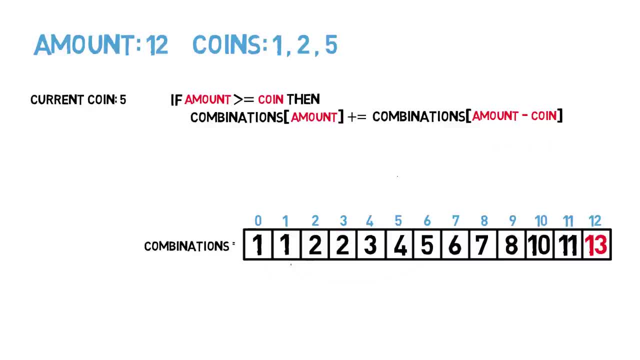 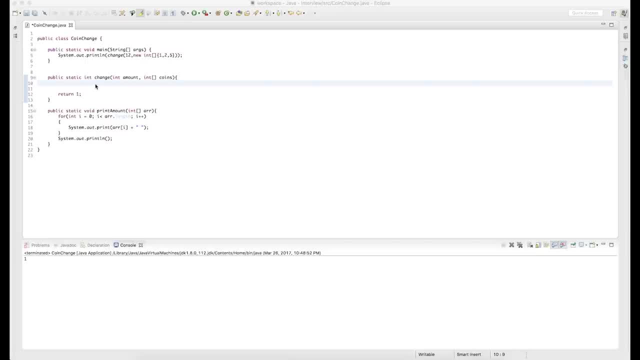 all you'd have to do is grab it from its location. So since we've gone through all that, let's write some Java code to implement this algorithm. So let's get started here. I already have this change method started. It has the input of amount and the array of coins. 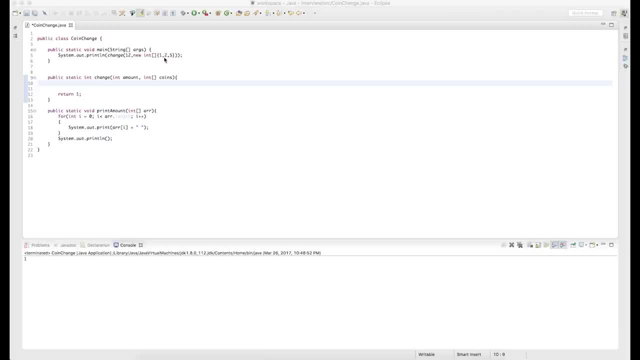 We are inputting twelve and then the coins one, two, five, just like the example. And now I have this helper method created. It's going to print out the amount for us. So let's start with the int array called combinations, new int. We're going to make it size, amount plus one. 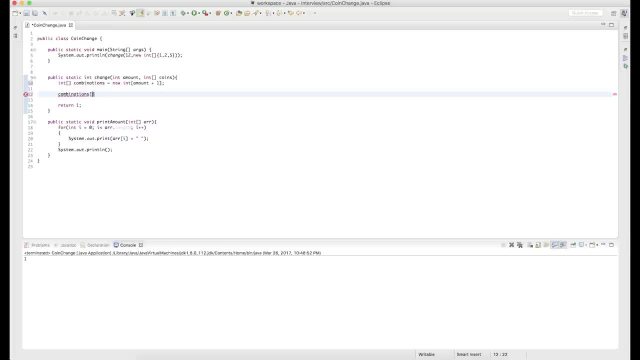 Then we're going to do combinations: zero equal to one. So now we need to iterate through all of these coins So we can do a for each. We're going to have an int coin through coins, So this is just going to go through each coin and select it as a coin. 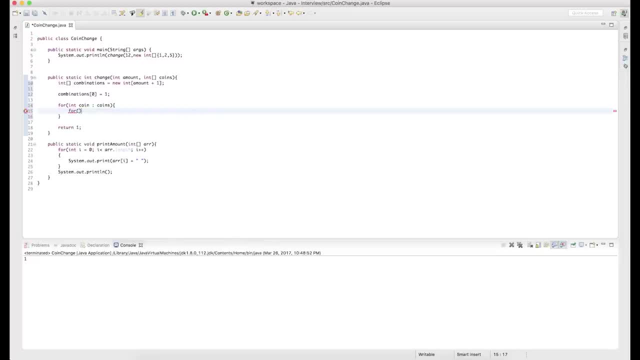 Now we need to go through this actual combinations array. So we're going to do int i equal to one, So we're going to start at one. Remember, we're not actually going to hit this, We're going to start at one and iterate through it from there. 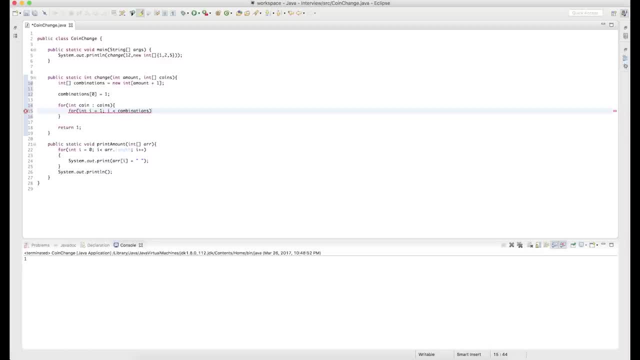 So we're going to do this. i is less than combinations dot length, i plus plus. So pretty simple. We're just iterating through the combinations array, But we're going to start at one. So we're going to do if i is greater than or equal to coin. 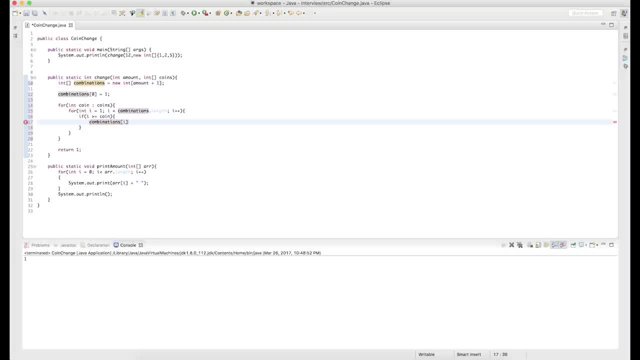 We'll do combinations. i is plus equal to combination i minus coin. So that's all you have to do. Well, we also have to change this to combinations amount to get the 12th spot in the array. So now it's going to go through each coin. 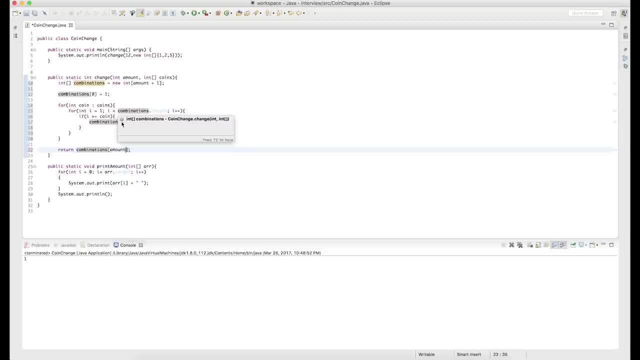 Then it's going to go through the entire combinations array. It's going to say: if that location is greater than or equal to coin, we're going to subtract it and then place it in that position. So let's run it. And we get 13,. just what we wanted. 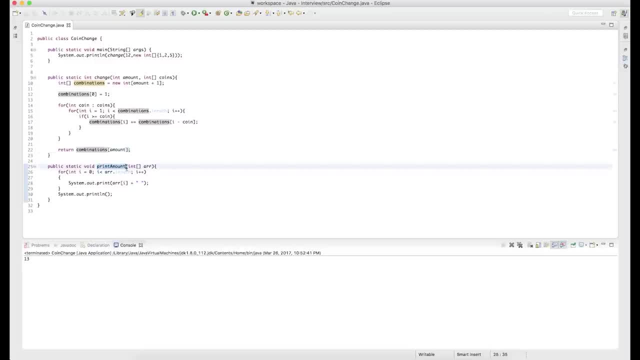 But if you want to see a little bit more of what's going on, let's put this print array right here. We're going to put combinations in there And I'll do a system dot out dot println to make it a little cleaner. 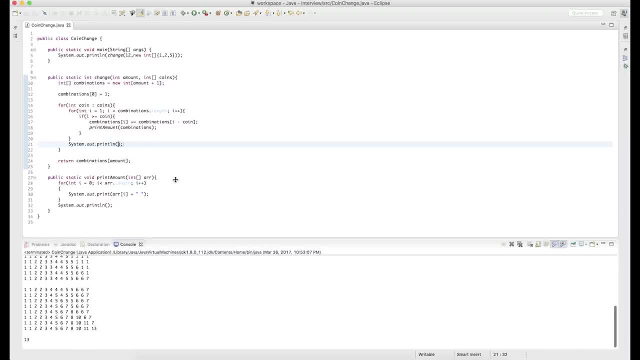 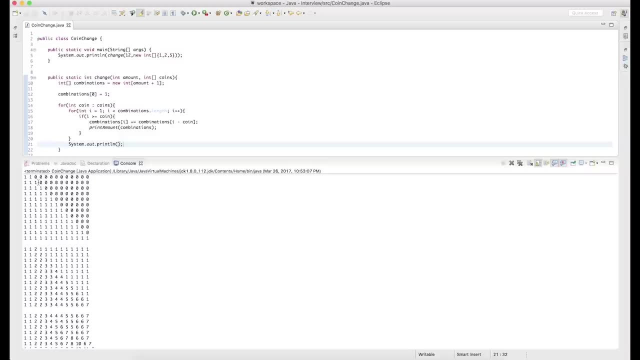 So let's run that, And this is just going to print out every step of the process. So it's going to start at 1.. It's going to go through. We're going to go here, look back, look back, just like I showed you before. 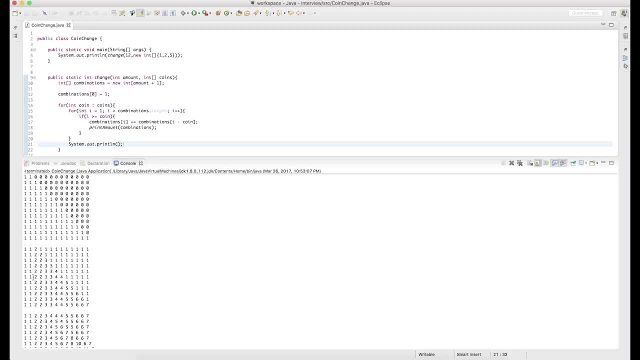 Then we're going to start at coin 2.. Coin 2 is bigger than this, so it's never going to change here And it's going to go through all the way to 7, just like we had Then for coin 5, it's going to go through. 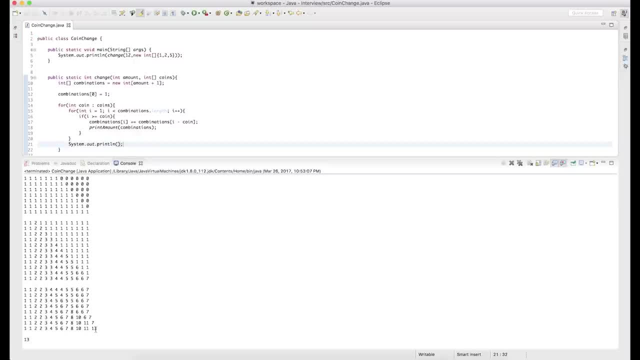 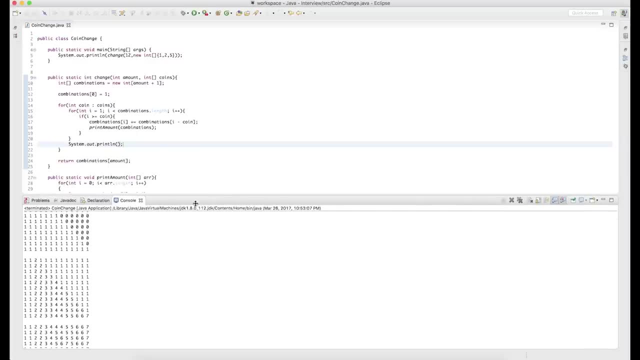 It's too big for these, so these are never going to change. It's going to go through And finally we hit the result of 13,. just what we wanted. So if you also wanted to, let's say you wanted coin 6,. 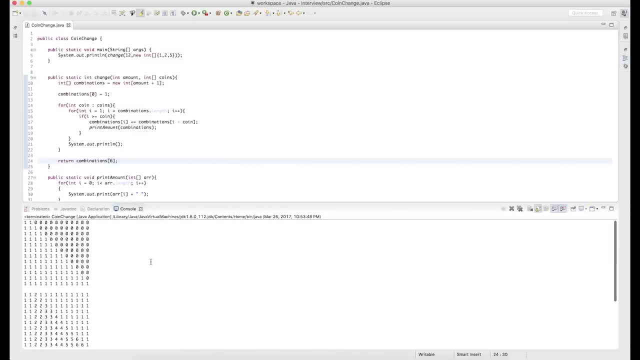 you could run that and you'll get the answer 5.. So right here. So you can put anything in here, as long as it's less than the amount. So there you have it. That's all you needed to do for this interview question. 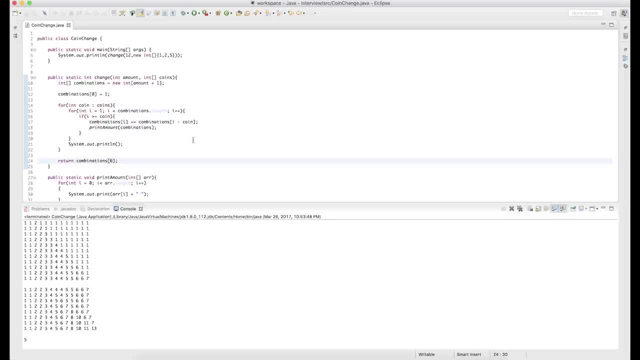 In the comments. let me know how I did. Let me know if there's anything you want me to do better. If there's any questions you want me to answer, let me know. Subscribe, and I appreciate it.